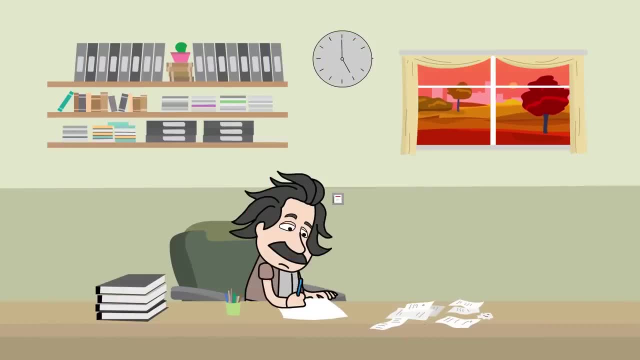 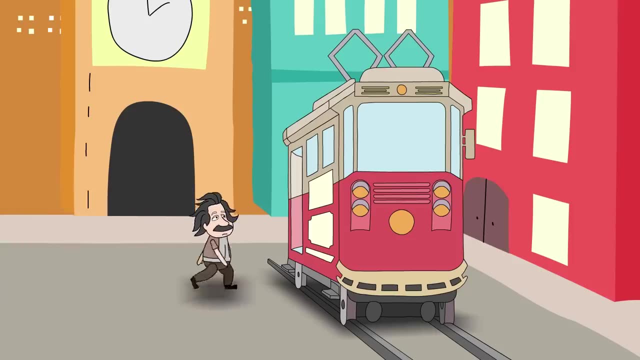 One evening in the spring of 1905, Albert Einstein, then a mere patent clerk in Bern, after trudging through his day's work, decided to board a tram car on his way home. Einstein would often wrap up his work as soon as possible to contemplate the truths of the. 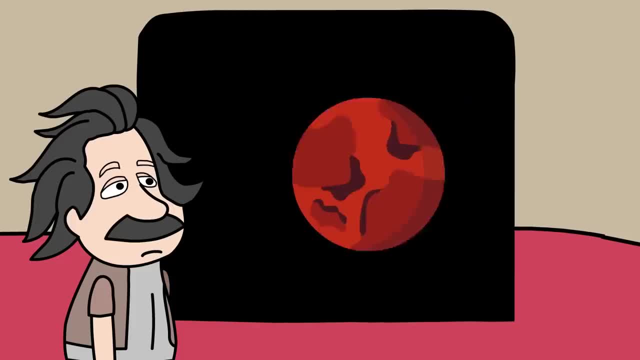 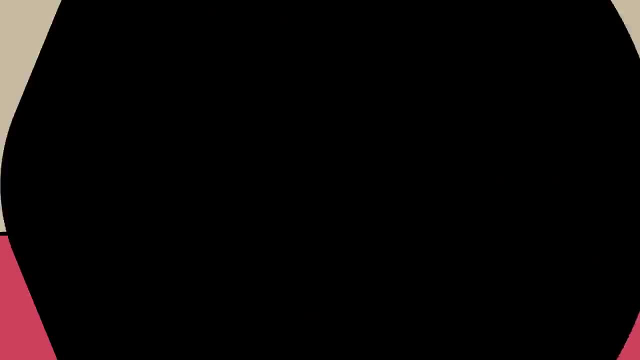 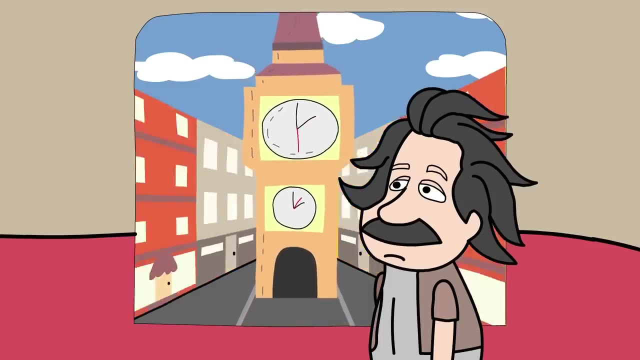 universe in his free time. It was one of these thought experiments he devised on that tram car that revolutionized modern physics forever. While receding away from the zeitgeist clock tower, Einstein imagined what would happen if the tram car were receding at the speed of 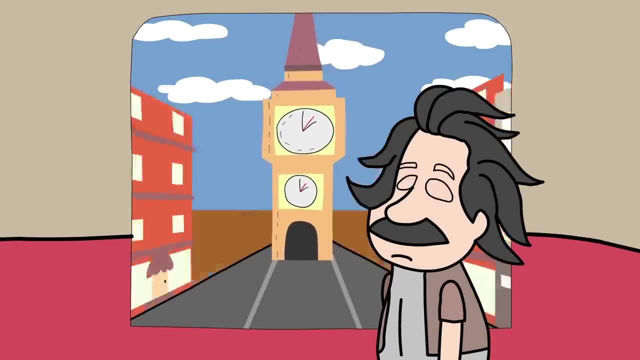 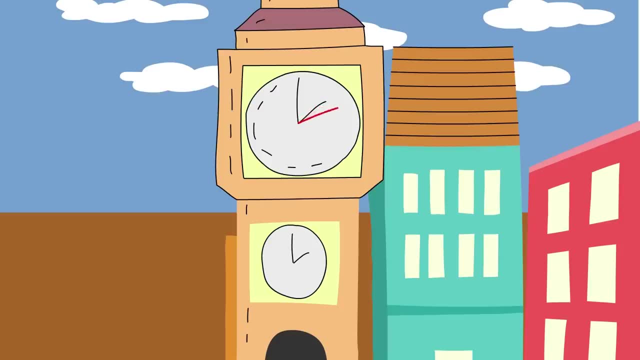 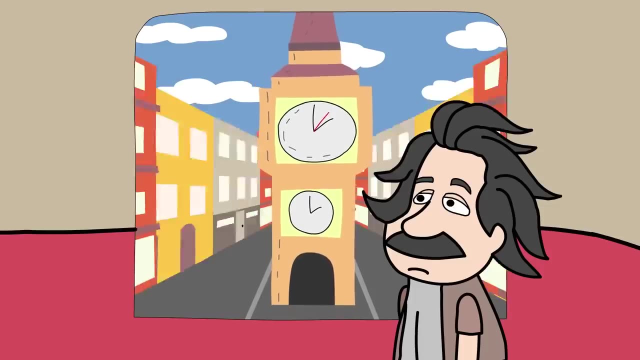 light. He realized that if he were to travel at 186,000 miles per second, the clock's hands would appear to completely freeze. At the same time, Einstein knew that back at the clock tower, the hands would tick along at their normal pace. For Einstein, time had slowed down. 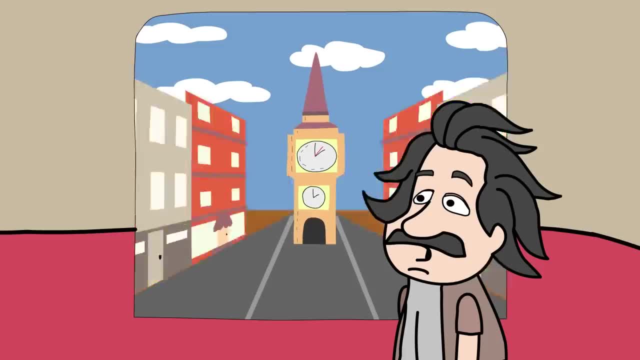 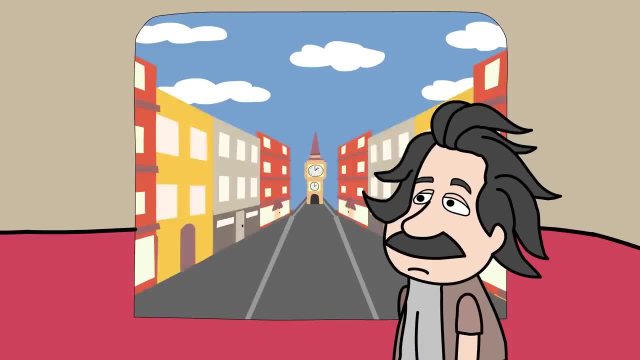 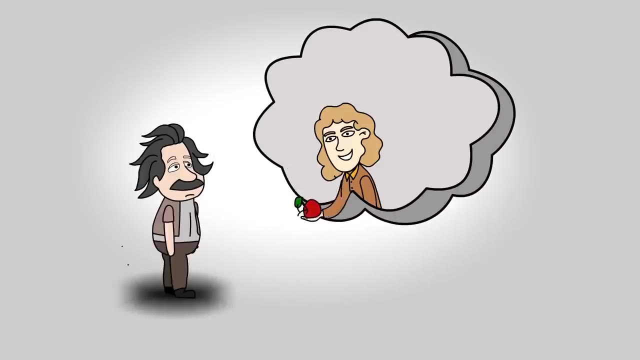 This thought blew his mind. Einstein concluded that the faster you move through space, the slower you move through time. How is this possible? Einstein's work was heavily influenced by two of the most iconic physicists of all time. First, there were the laws of motion, discovered by his idol, Isaac Newton. 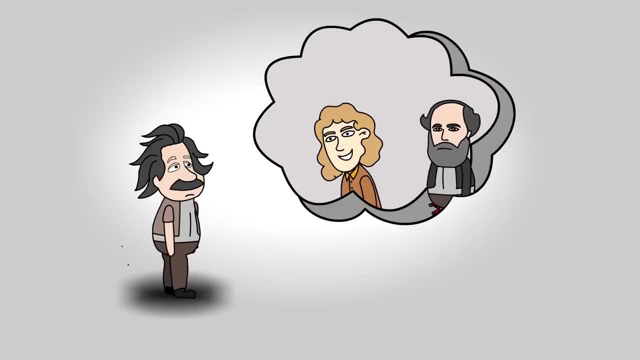 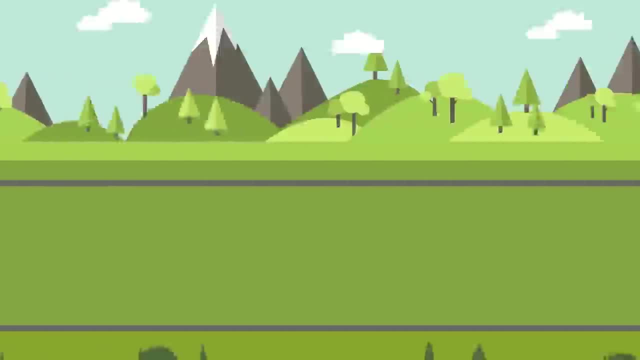 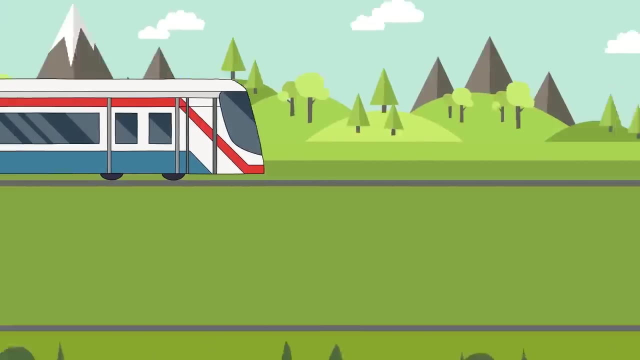 and second were the laws of electromagnetism laid down by James Clerk Maxwell. Newton's laws insisted that velocities are never absolute but always relative, so that their magnitudes must be appended by the phrase with respect to, For instance, a train travels at 40 kilometers per hour. 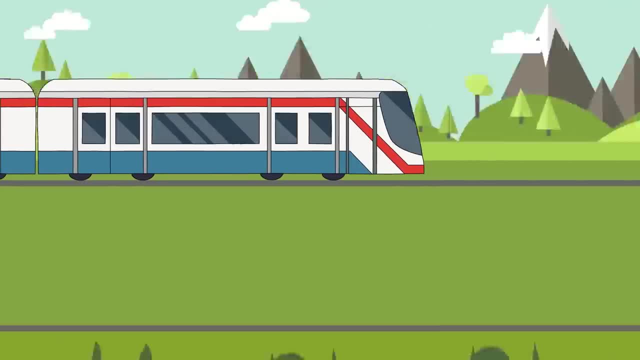 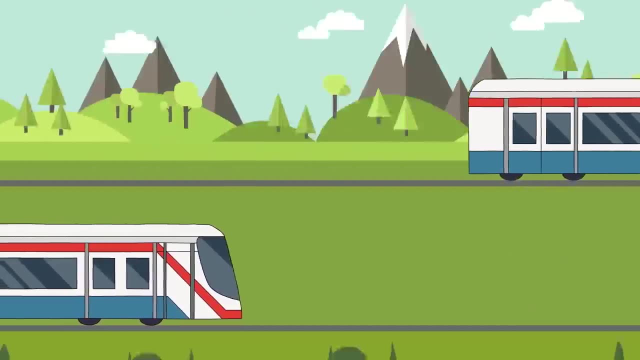 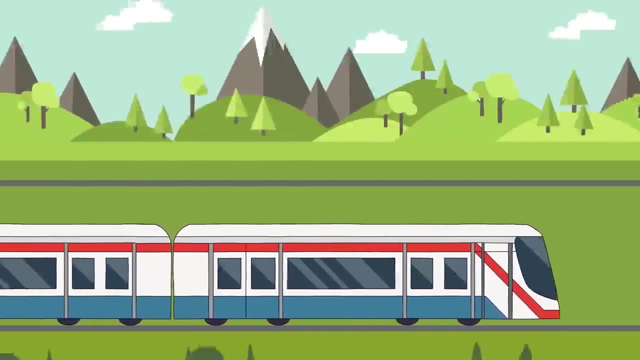 with respect to someone at rest. However, it only travels 20 kilometers per hour with respect to a train traveling 20 kilometers per hour in the same direction, Or it travels 60 kilometers per hour with respect to another train traveling in the opposite direction at 20 kilometers per hour. 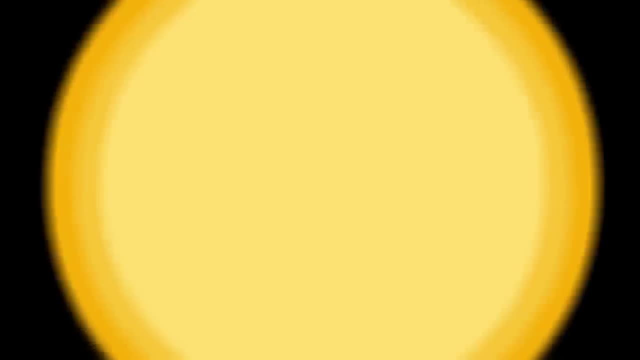 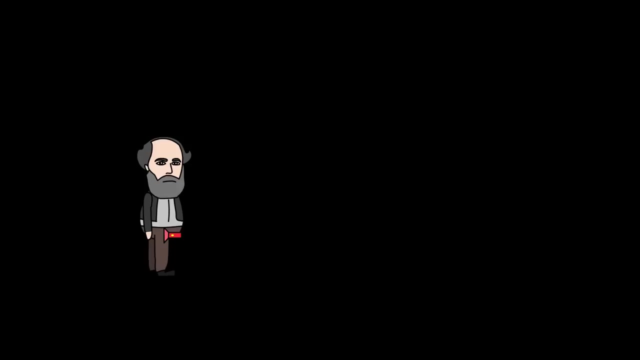 This is also true for the velocities of Earth, the Sun and the entire Milky Way galaxy. On the other hand, Maxwell found that the speed of an electromagnetic wave such as light is fixed at an exorbitant 299,792,458 meters per second. 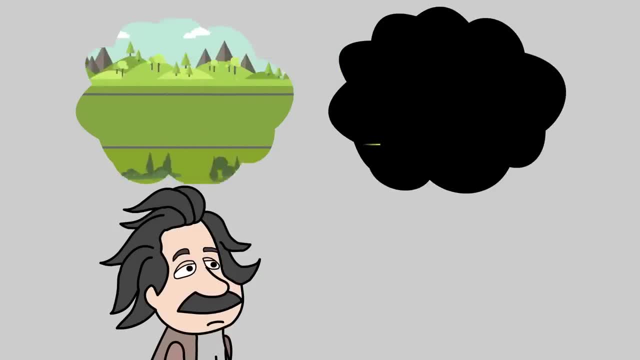 regardless of who observes it. However, Maxwell's notion seems incompatible with Newton's notion of relative velocities. If Newton's laws are truly universal, why should the speed of light be a constant? Why should the speed of light be a constant? Why should the speed of light be a constant? 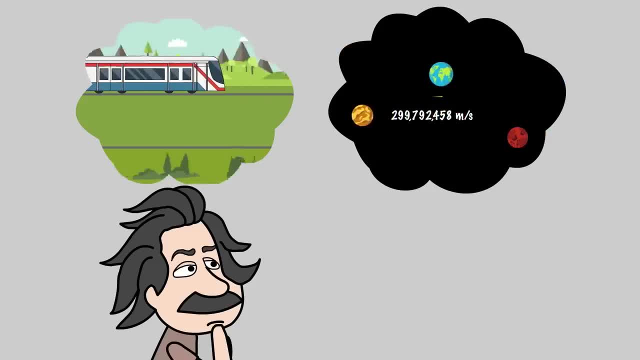 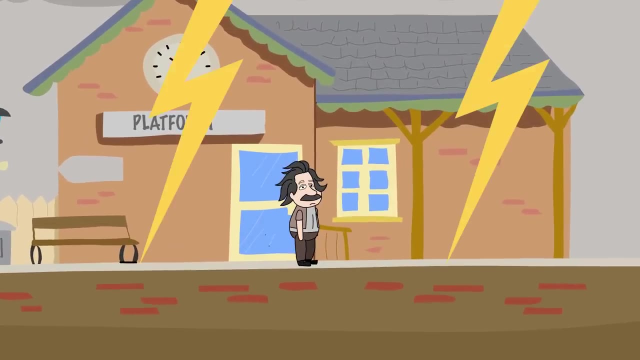 This presented Einstein with a daunting dilemma. This conflict between the ideas of Newton and Maxwell can be demonstrated with another of Einstein's brilliant thought experiments. Einstein imagined himself on a train platform witnessing two lightning bolts strike on either side of him. Now, because Einstein stands precisely- 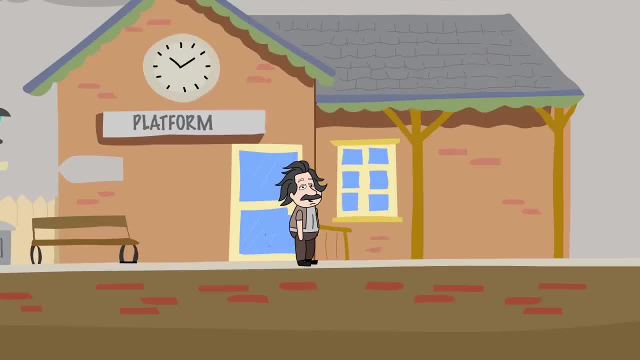 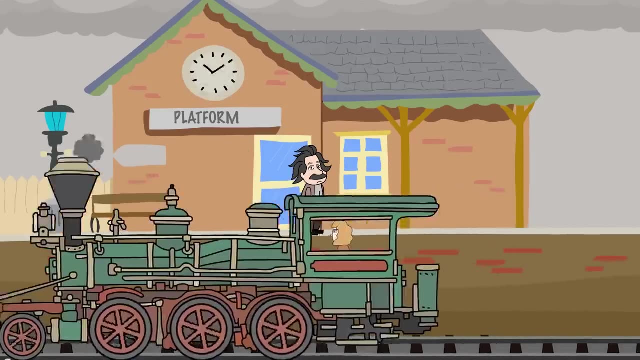 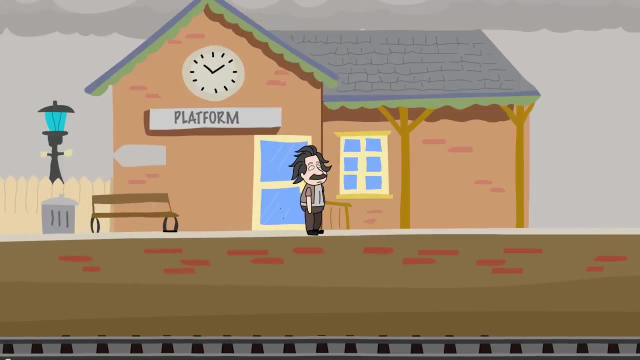 in the middle of the two strikes, he receives the resulting beams of light from both sides at the. However, things get more complicated when someone on a passing train views this event while whizzing past Einstein at the speed of light. If the speed of light conforms to the rules of relativity, then the person on the train 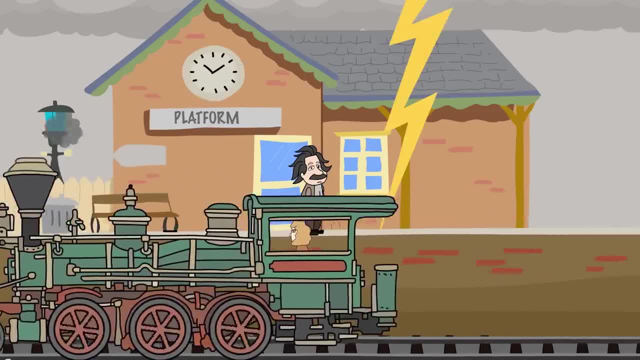 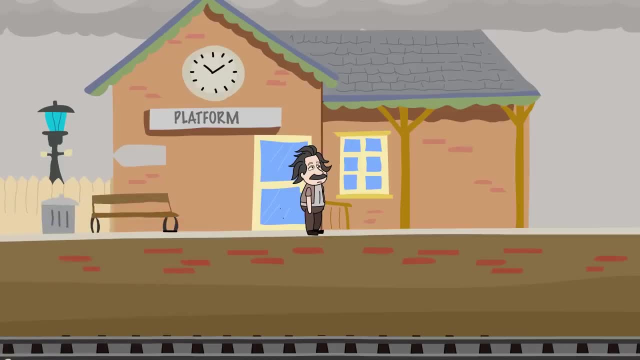 wouldn't witness the lightning strike simultaneously. Logically, the light closer to the man on the train would reach him first. A measurement of the speed of light made by both men would differ in magnitude. This would contradict an apparently fundamental truth of the universe. 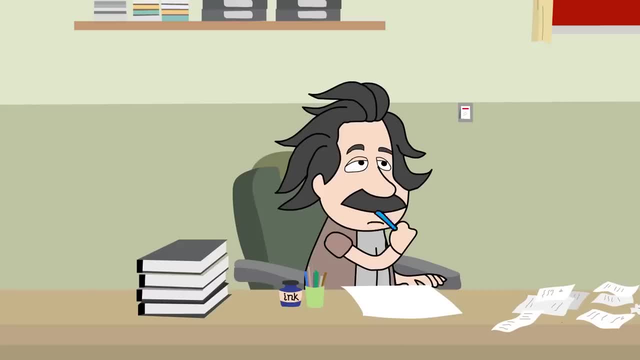 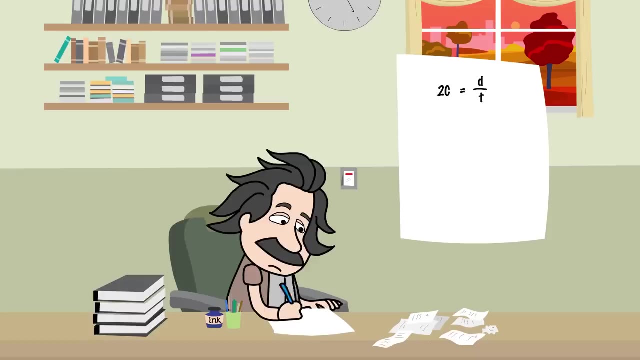 Einstein had to make a difficult choice: Either Newton's laws were incomplete or the speed of light was not a universal constant. Einstein realized that the two notions could coexist with a small tweak in Newton's laws To get rid of the discrepancy in the measurements. Einstein suggested that time itself for the 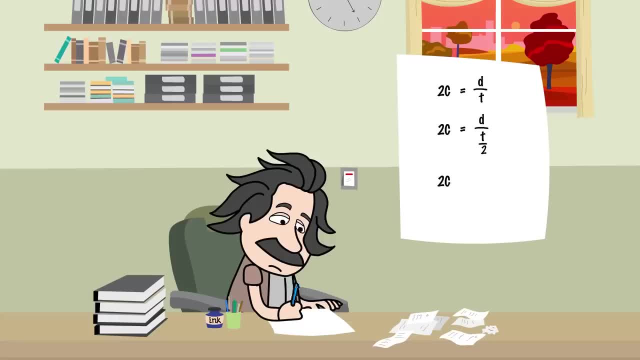 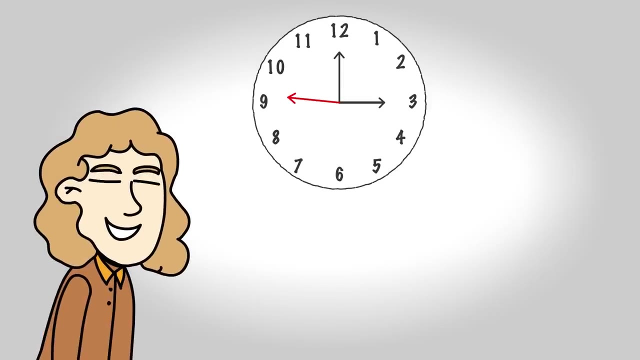 man on the train must slow down to compensate for the decrease in speed, such that the magnitude remains a constant. Einstein called this absurdity time dilatation. Newton believed that time moved unflinchingly in a single direction forward. Einstein, however, had just realized that time stretches and contracts varying with 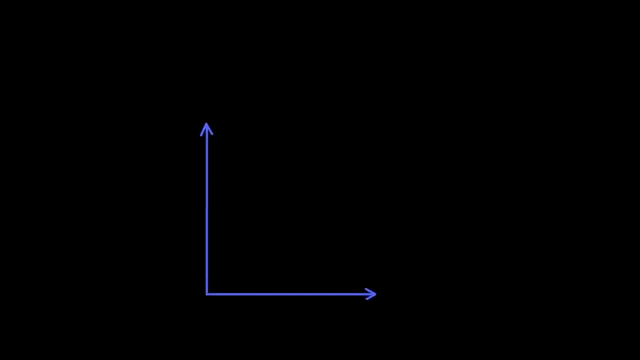 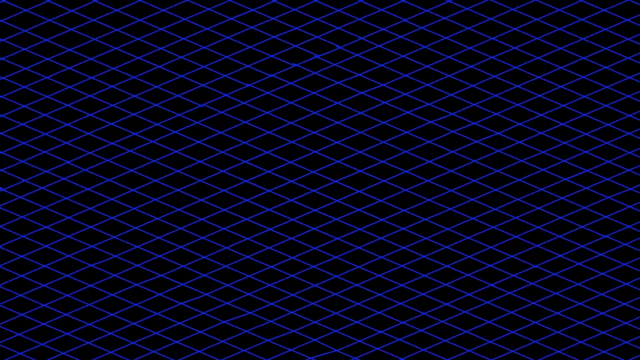 velocity. Due to its malleability, time, like space, deserved its own dimension. In fact, Einstein claimed that the two were one and the same. Together they formed a four-dimensional fabric, A continuum called space-time, upon which the mundane events of the universe would unfold. 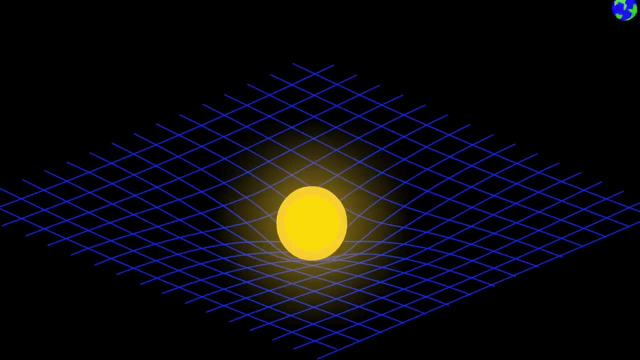 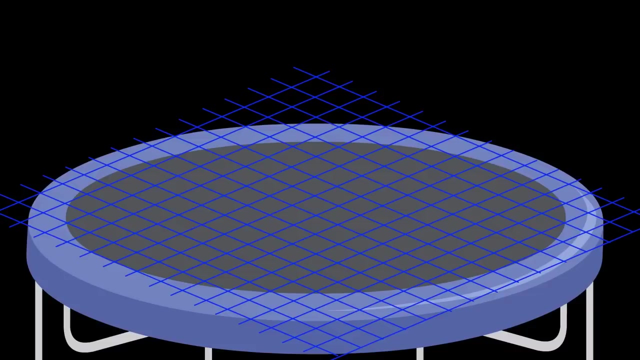 Einstein suggested that massive objects like the sun didn't pull bodies like Earth with a mysterious, inexplicable tug, but rather curved the fabric of space-time around them, forcing Earth to fall down into this steep valley. A highly simplified analogy is the dip in a trampoline made by the tip of a bowling. 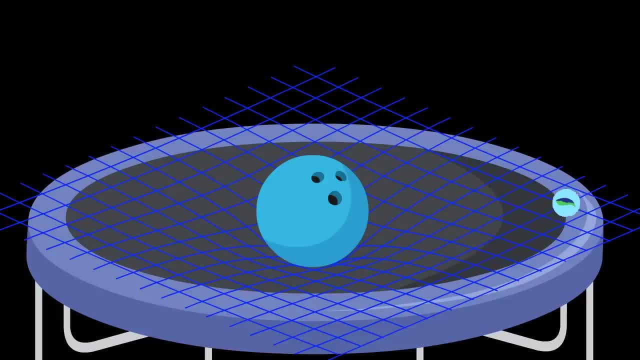 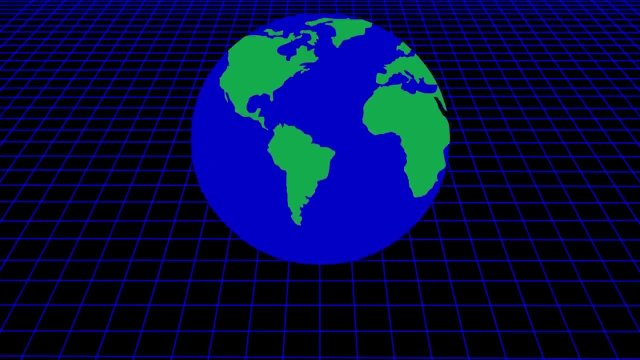 ball. If we were placed on that trampoline, the marble would immediately roll towards the bowling ball in the center. This is also true for Earth's gravity. We are pinned to the ground because space so distorted by the Earth's mass pushes. 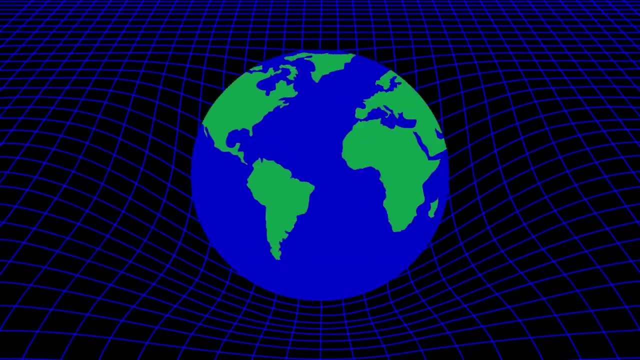 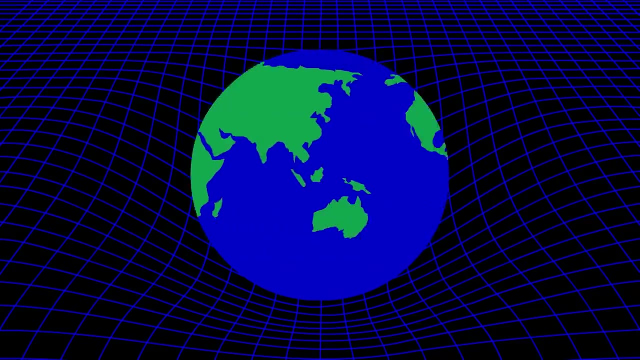 us down from above. However, the slump in the fabric around Earth is not uniform, and Earth's gravity grows more intense as we move towards its center, where the curvature is at a maximum. Therefore, like the marble on the trampoline, an object that falls toward the center is. 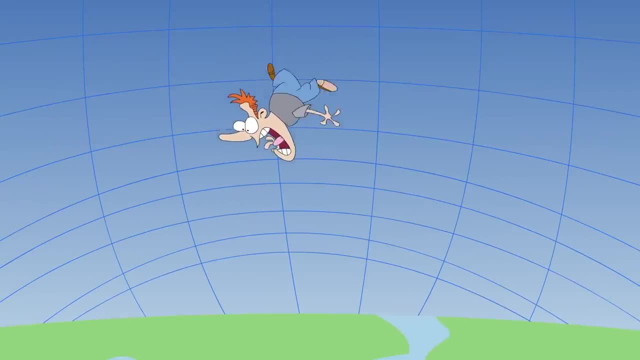 more likely to accelerate towards the Earth as it races towards the center of the planet. It falls faster when just above the surface than it does, say, when it is slightly above the atmosphere. But hey, according to special relativity, the faster you move through space, the slower. 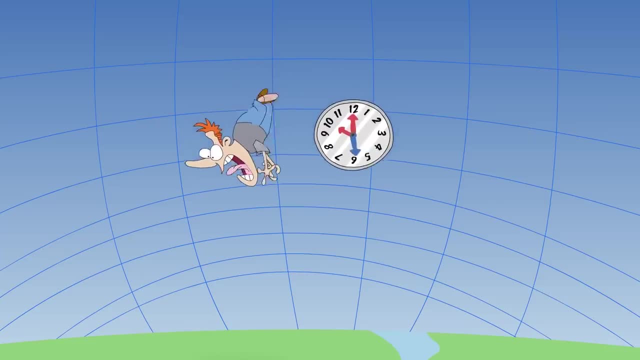 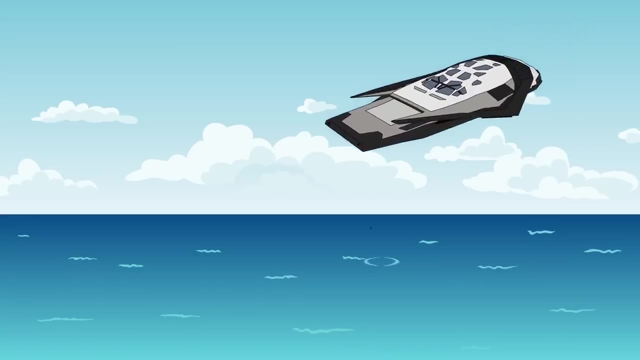 you move through time. This means that time runs slower on Earth's surface than it does above the atmosphere. Now, because different planets have different masses and thus different gravitational strengths, they also accelerate objects at different rates. As we have learned, this means a variable passage of time. 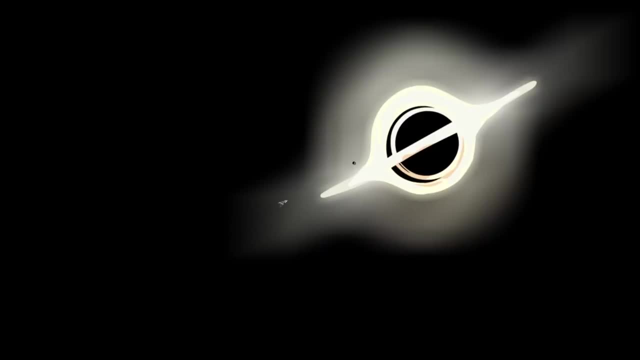 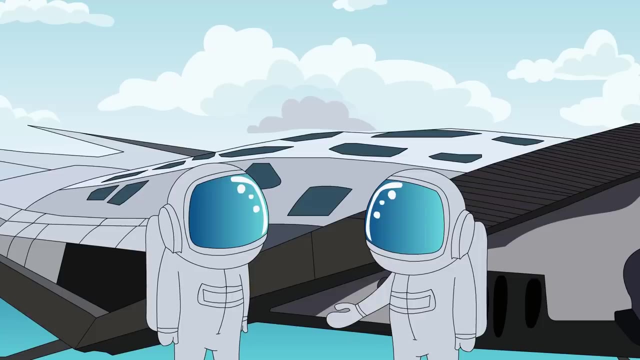 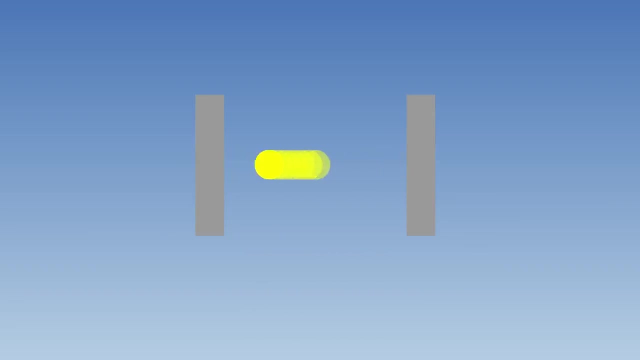 This is what happens in the movie Interstellar, when the protagonists land on a planet in the proximity of a black hole. The gravity on the planet is so severe that one hour on the surface is equivalent to seven years on Earth. To understand how motion affects time, let's consider the simplest timekeeping mechanism. 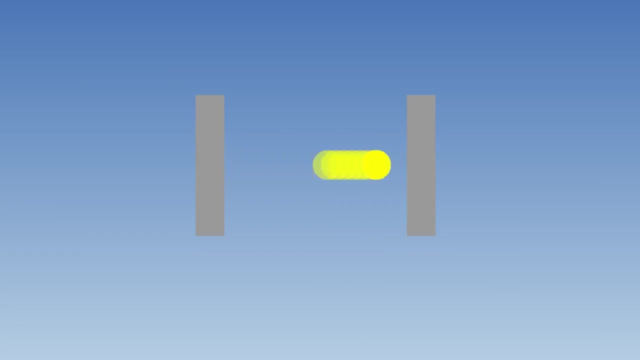 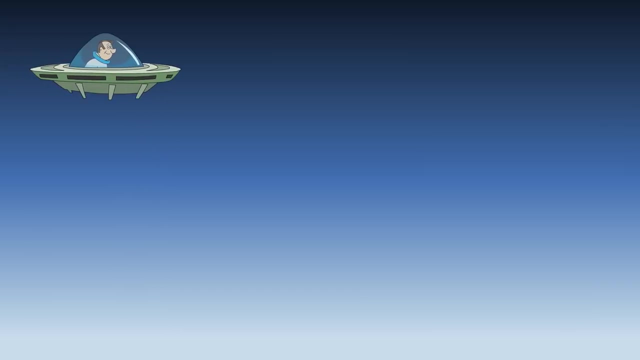 Time is divided by time. A second passes each time time the photon enters the model- This is also known as a acceleration- is reflected. Let's imagine two people: one in a spaceship slightly above Earth's atmosphere and the second on top of a small hill just above the Earth's surface. Both are watching a man fall. 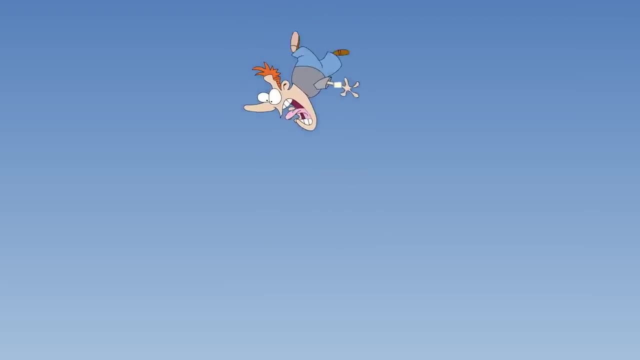 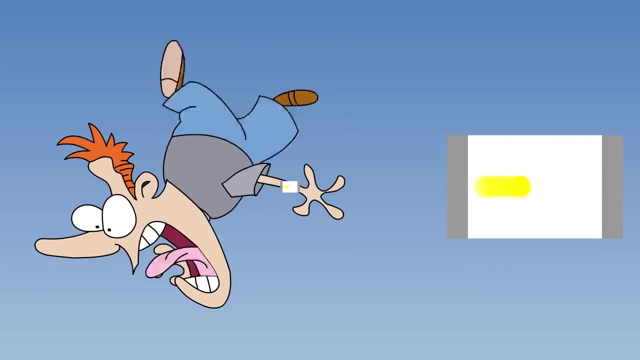 from space towards the ground. Let's say that the falling man is carrying the photon clock explained a moment ago. What do each of the two men observe as the man falls past them? What they observe is eerily similar to what a stationary person would observe when watching a ball bounce in a moving